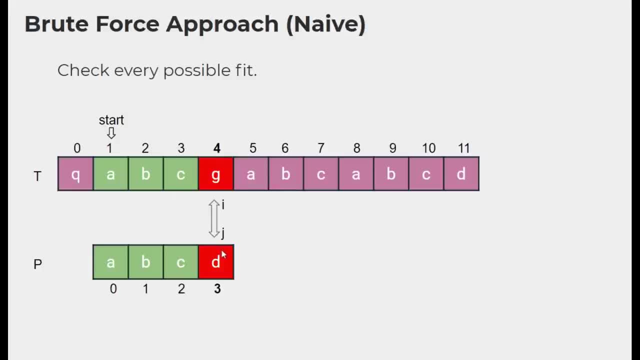 match. and when we find a mismatch later in the pattern, like this: See here the index of the pattern is 3 and we find a mismatch here. We have actually started our comparison from the first index. Now, since we have a mismatch, we move back i to the second. 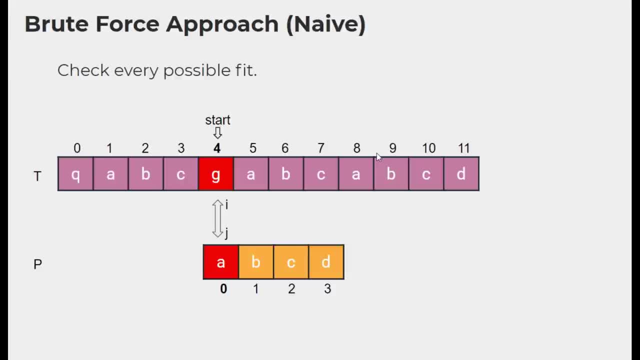 index and start comparing from this position. We continue doing this until we reach the end of the text. Consider this worst case example of brute force. Whenever there is a mismatch, the text pointer is moved backwards and we are doing a lot of comparisons. Clearly, brute force is not doing. 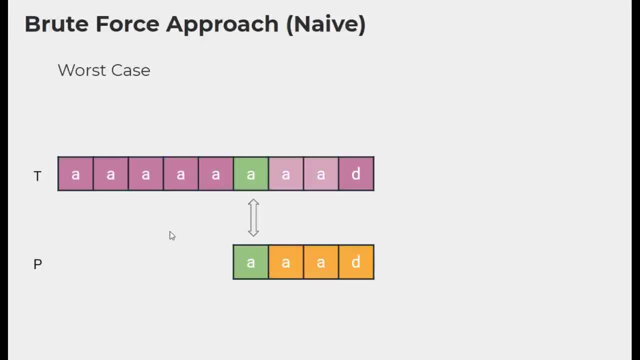 well, when we have more repeated characters like this in both the text and the pattern- Say, the text is of length n- In the worst case scenario, what do we do is we first start with here and do m comparisons, and then we start here and do another m comparisons. So we keep doing this until this point. 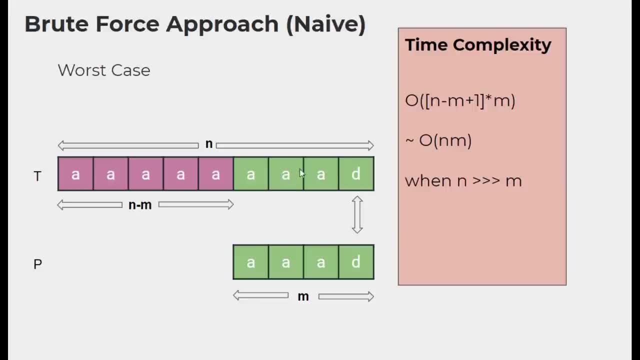 because there is no point in starting from this position. The pattern will anyways be truncated. So this is the final starting point, which is n-m plus 1.. For each of these n-m plus 1 characters, we are doing M comparisons. So the worst case- complexity- is this. Analysis of time. complexity itself comes. 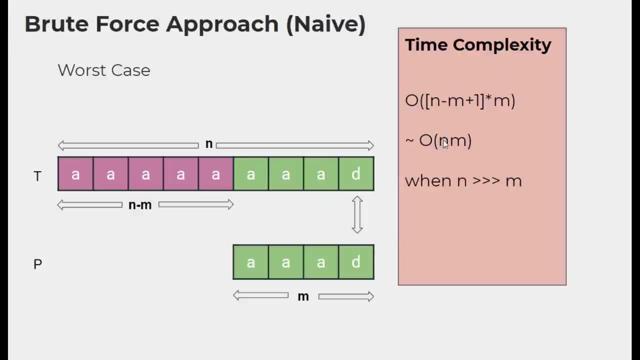 into picture only for very large inputs, right? So N is obviously going to be very large when compared to M, the length of the pattern. So this can be considered as O of N into M. We can ignore the M square and the M terms since they are going to be very small. Before directly jumping, 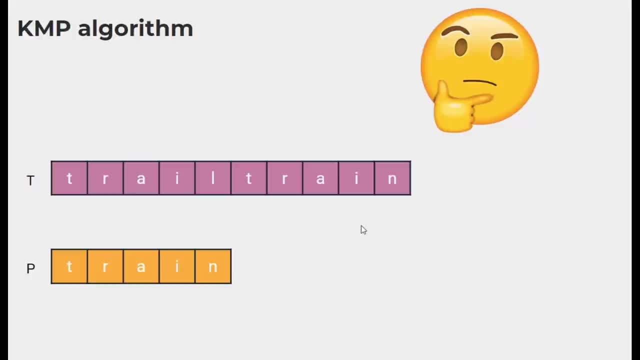 into the algorithm. let's first think how to improve the brute force technique. Consider this easy example. We find that the first four characters match and the last character is a mismatch With brute force. we go backwards and start comparing from this position, This going. 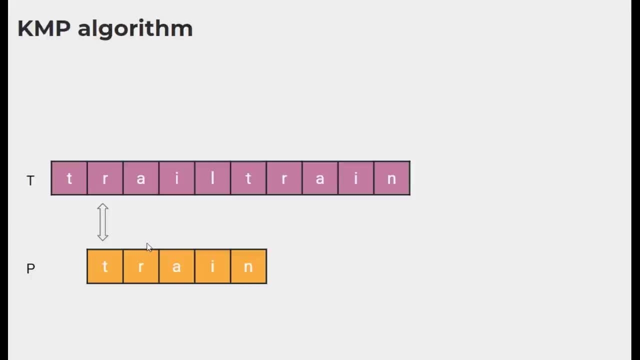 back is what is making the brute force approach very slow, right? So how can we avoid going backwards When we find a mismatch like this? we know that the previous characters match right. In this example, the previous four characters of the pattern matches with the previous four. 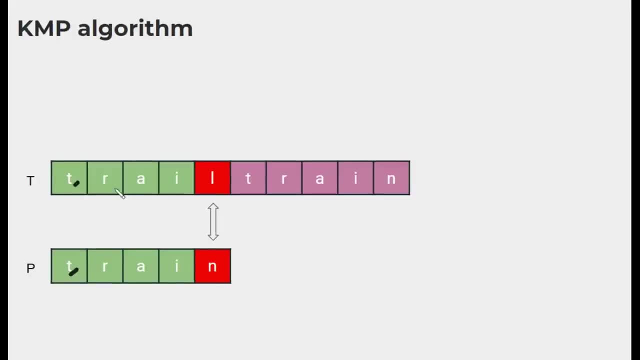 characters of the text. We know that this and this match, this and this match, then what's the point in going all the way back and trying to compare this with this? So instead of going backwards like this once we find a mismatch, can we just start comparing? 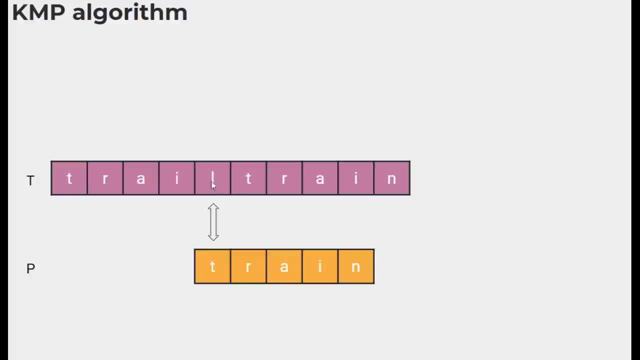 the pattern from this position, from where the mismatch was found, ignoring altogether all the previous characters of the text. Let's see, It seems to work in this example. Here is a mismatch, So we move forward and we are able to match the entire string here. But this definitely is not. 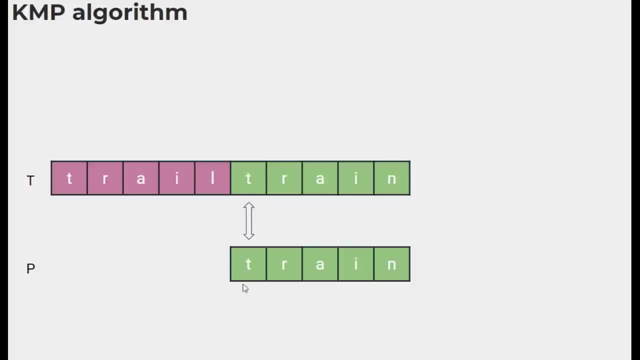 the right approach. It is working in this example Because all the characters in the pattern are distinct. Consider this example now. The first five characters match and there is a mismatch here in the last character If we go by our previous technique, that is, if we just ignore all the previously matched characters and just 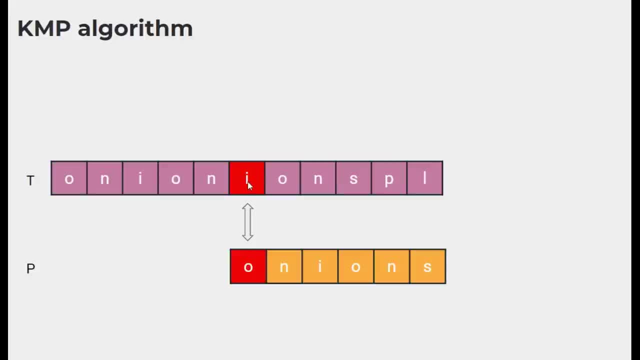 start comparing from this mismatched position. just like this, we will not be able to find the required pattern, which is actually present here. We will be missing it. By totally ignoring the previously matched characters, we will be missing the pattern. So let's see. 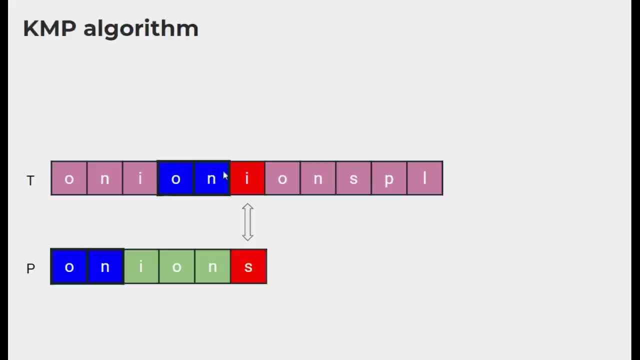 We are missing the overlapping characters like O and N in this case. So how exactly do we find these overlapping characters? We know that the previous five characters of the text, as well as the pattern, match when there is a mismatch in the sixth character of the pattern, right With this. 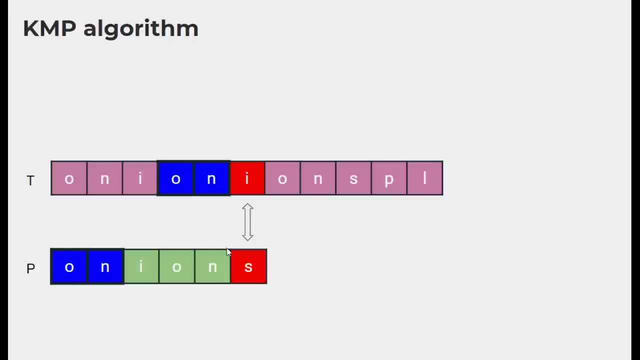 information. just consider this particular substring, the first five characters. We know that the exact same five characters are present previously in the text, right? So in this case we can look at the prefixes of the pattern and we can match them with the suffix of the text. 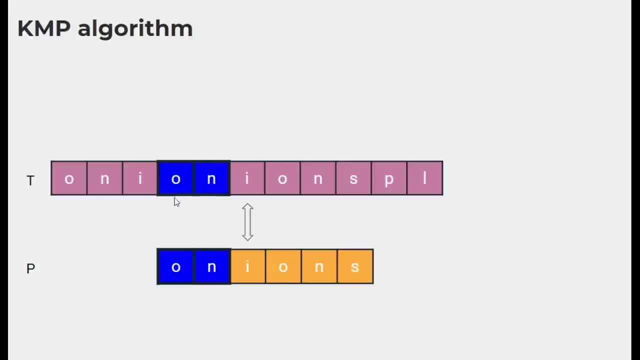 So we can skip all the previous comparisons and start comparing from this third position, or exactly the second index of the array. Moreover, it is not just some prefix, that is also a suffix. It should be a longest prefix. that is also a suffix. Only then we can correctly match them. 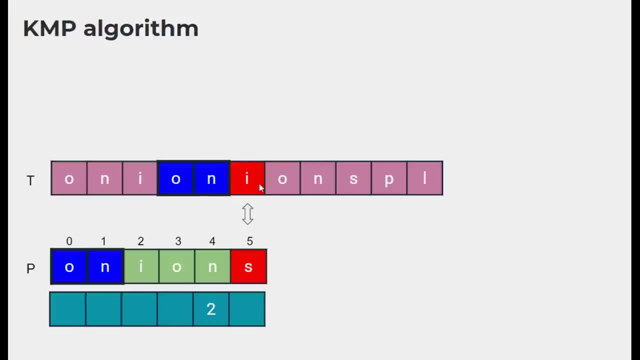 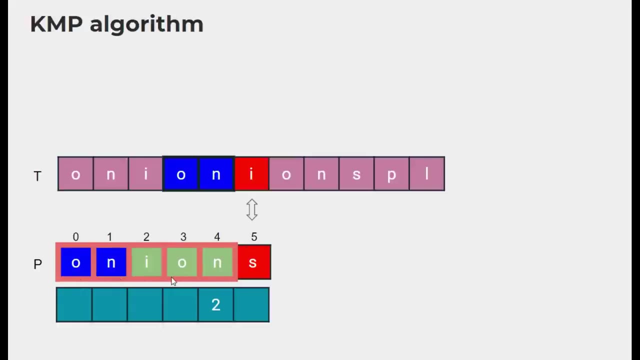 and skip maximum comparisons. Here we have the mismatch in the fifth index of the pattern right, which means the index 0 to 4 exactly matches with the previous characters of the text. so now consider only this substring. in this substring, the longest prefix, that is also a. 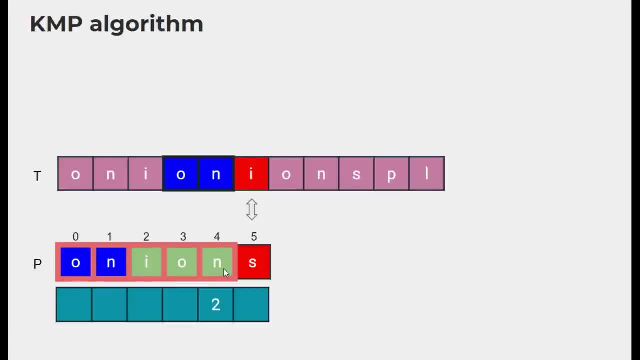 suffix is of length 2. if we pre-calculate this information for each index of the pattern and store it in an array, that is, until that particular index, what is the length of the longest prefix? that is also a suffix. if we have that information readily, we can easily look up this table and 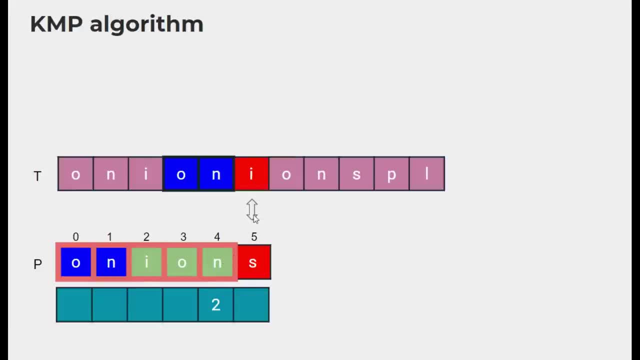 determine what is the next position that we have to compare whenever a mismatch occurs. in this example, the mismatch occurs in the fifth index, which means until the fourth index all the characters have matched. and if i go to the fourth index of the table and if it tells me what is the length, 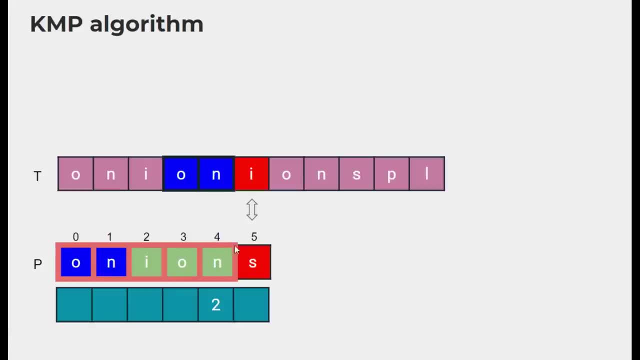 of the longest prefix- that is also a suffix- until fourth index, that is in this case if it says 2. if i have that information, i will understand that the characters in the zeroth and the first index are already matching, so it's enough. if i start comparing from the second index, i can skip all these. 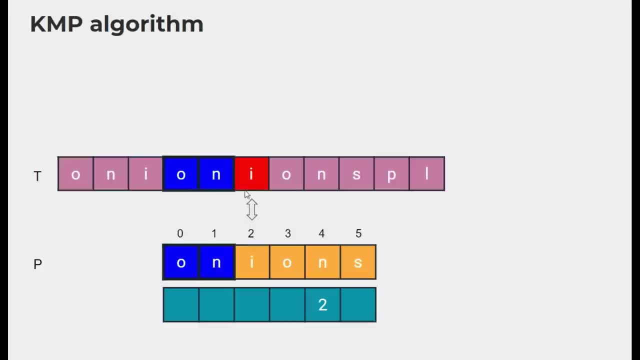 comparisons. without moving this pointer for the text, we are able to now determine from which position in the pattern we should begin our comparison. so this is what is the logic behind the kmp algorithm: you are just pre-calculating a table which tells you, for each index, what. 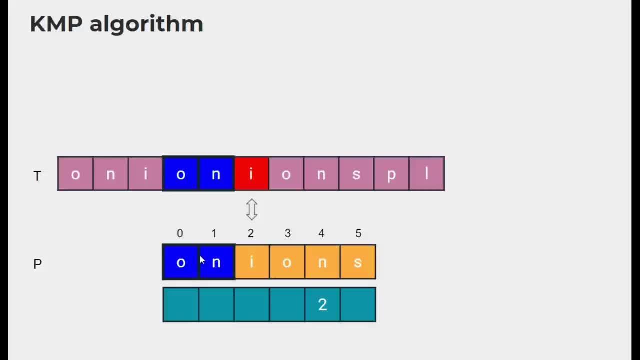 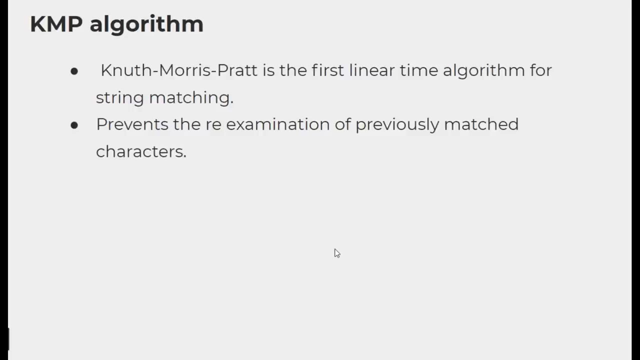 is the longest prefix. that is also a suffix until that point. so when you are searching through the string, whenever a mismatch occurs, you just can look up that table and determine from where you should start comparing in the pattern, without even moving the text pointer. this algorithm was developed by 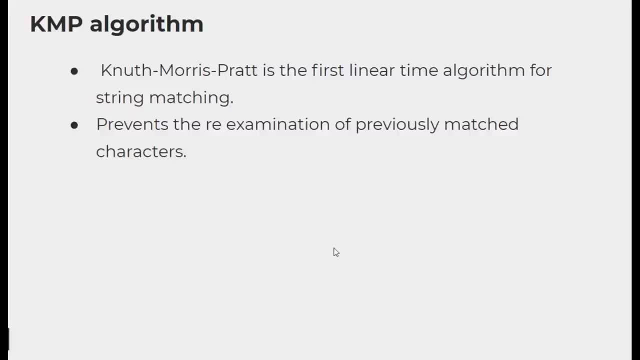 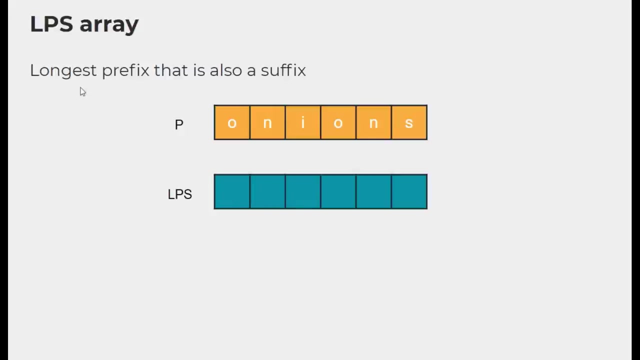 newt, morris and pratt independently, and it is the first ever linear time algorithm for string matching. unlike brute force, it totally avoids the re-examination of the previously matched characters. so that's why, when you consider that there is a mistake in the number of characters in here, 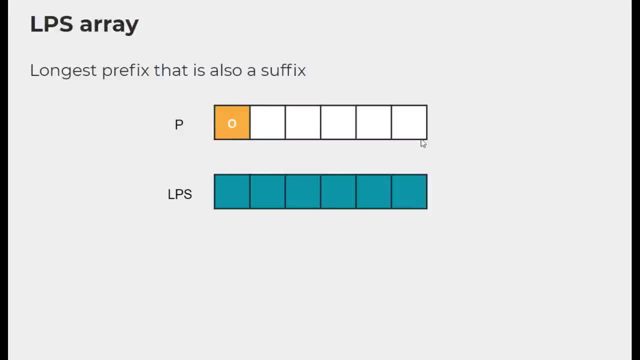 here. for example, let's try to fill up the entire lps array. lps stands for the longest prefix. that is also a suffix. when you are calculating for the zeroth index, just forget about the remaining part of the array: the length of the longest prefix. that is also a suffix for this particular. 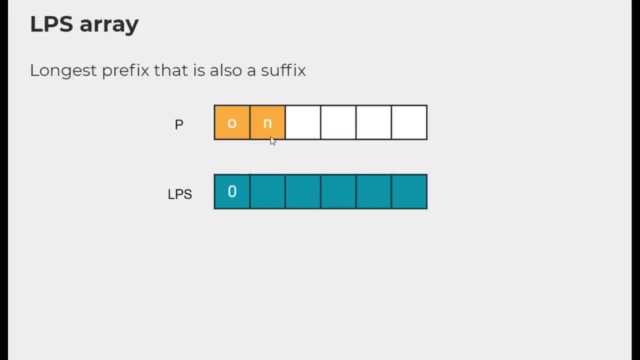 character will be zero. right, while calculating for the first index, you have to take the first two character into consideraation. here again, they are not equal, So that's why we have a 0.. If you take ONI, again, it will be 0.. If you have 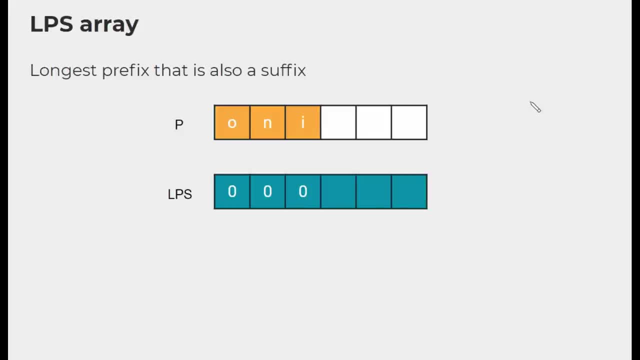 trouble in understanding this. just write down all possible prefixes and the suffixes for this substring. For ONI, O is a prefix, ON is also a prefix. Similarly, I is a suffix. NI is also a suffix. None of these match. There is no prefix. that is also a suffix. So that is why we have 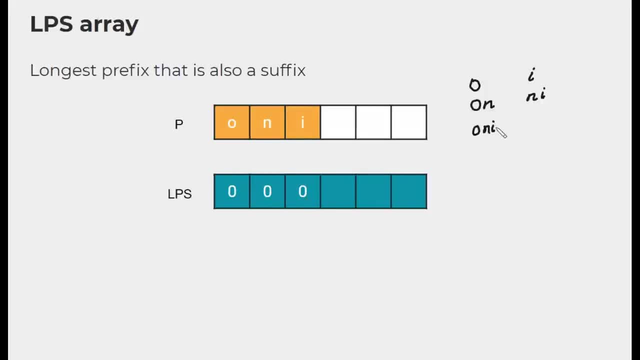 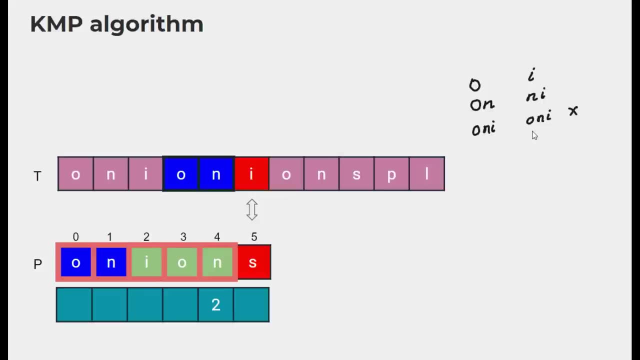 a 0 here. Don't take ONI as a prefix and ONI also as a suffix. This cannot be done. Why I cannot consider ONI as a prefix as well as a suffix. See here: ONI ON is a substring. 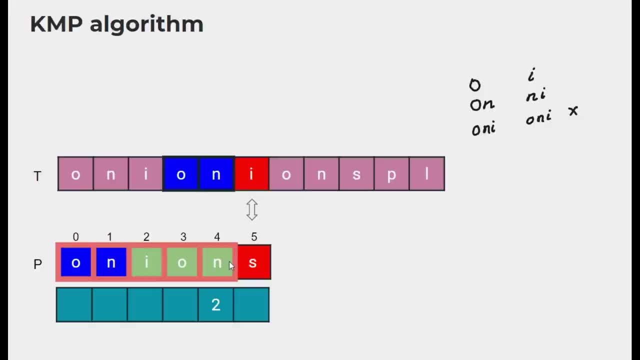 I can very well consider that as a prefix as well as a suffix, But then I have to start comparing from this position. I already know that this position does not match The logic of computing. this LPS array itself will be meaningless if I take the entire substring as prefix. So 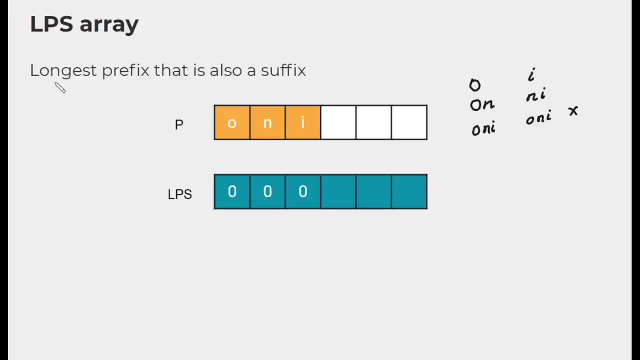 that's why I have to start comparing from this position. That's why we are not doing that. We also commonly say the longest proper prefix. that is also a suffix. By proper we mean this only, That is, we cannot consider the entire substring as a. 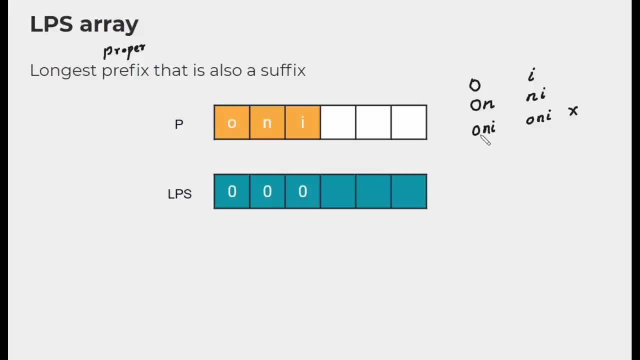 prefix. Anything less than that is only a proper prefix. Now, when we consider the first four characters, O is a prefix and it is also a suffix. That is the longest prefix that we can find. That is also a suffix. So here we compute: 1. Taking the first five characters ON is a prefix. 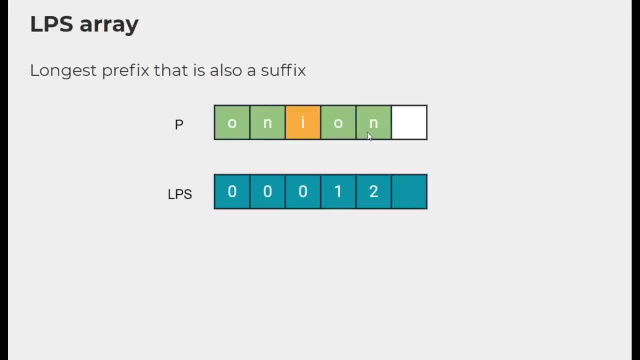 and it is also a suffix: The longest possible prefix and suffix. So we have two here. Now, considering the entire pattern, again there is no prefix. that is also a suffix. I have just written down all possible prefixes and the suffixes. Nothing matches. So here again we have 0. 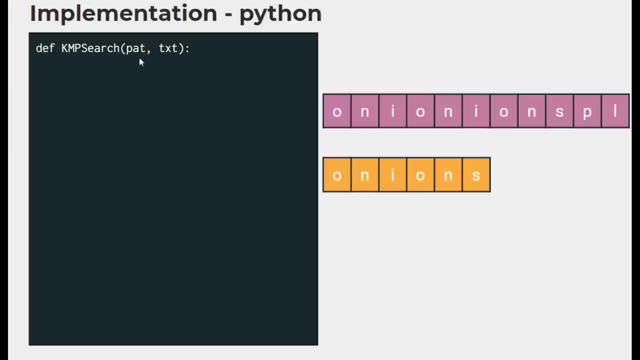 Let's see the implementation with Python. For the search function we receive the pattern and the text as the parameters. First we compute the length of the text and store it in N, and then length of the pattern is stored in M. We need to compute the length of the text and store it in N. 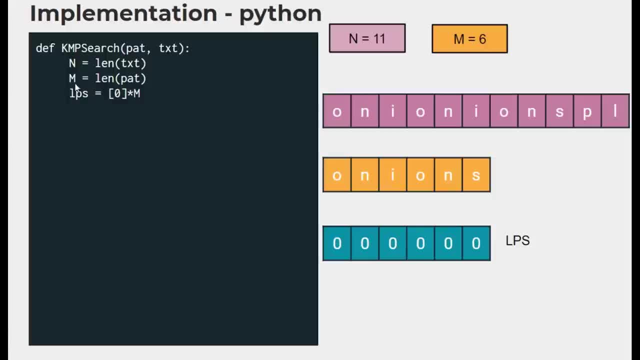 We need to compute this LPS array. It should be of same length as the pattern, So we are initializing it with M zeros. We make use of a separate function to calculate the LPS. Let's get to the implementation of this function later in the video. First, let's finish off this search. 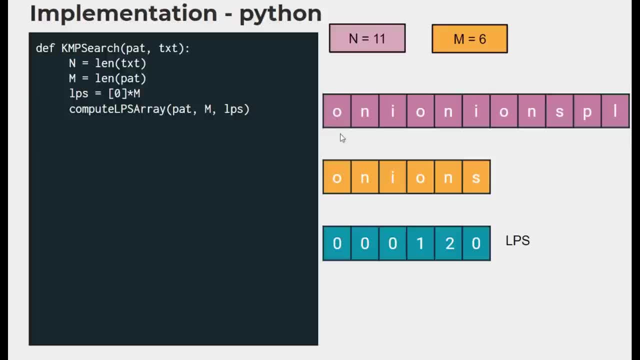 part. So during search we have to compare, starting from the beginning, index of both the text and the pattern right. So we need to have two different pointers for the pattern and the text. So we have I and J and we are initializing them as 0, since we have to start from the beginning. 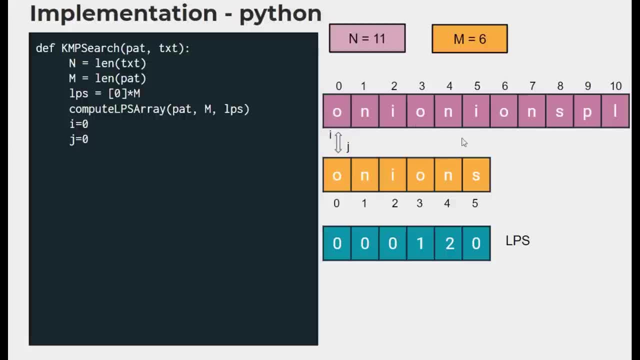 We need to scan through the entire text input to find the pattern. So the loop runs until N, the length of the text. First we compare these two characters and if we find a match, what are we supposed to do? We just have to increment both the pointers, right? 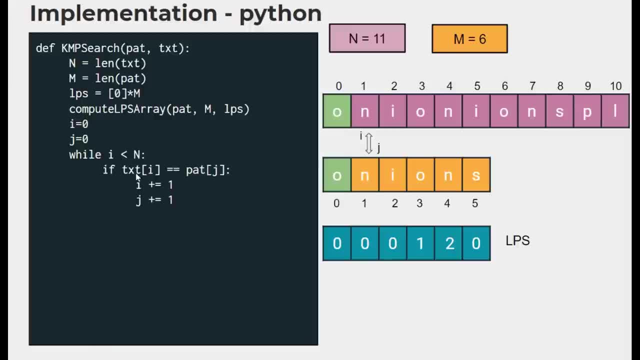 So let's have that in an if. If the character at the text and the pattern matches, then we just have to increment both the pointers. The next four characters also match. So we keep incrementing the pointers and there is a mismatch in the fifth index. When there is a mismatch, we have to. 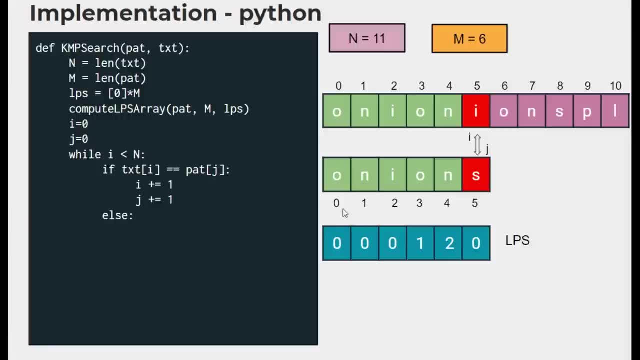 match in the fifth index of the pattern. We know that the index from 0 until 4 is a perfect match. So if we go to the LPS table and check what is the value at the fourth index of the table, it will tell us the length of the longest prefix. that is also a suffix until this point. 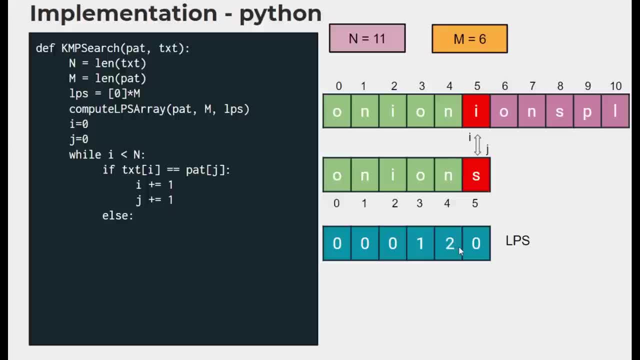 until the fourth index. It says 2.. 2 indicates the length of ON. ON is the prefix and it is also a suffix. So when we see a 2 here, we can understand that the characters at the 0th and the first index are already matching with the previous characters of the text. 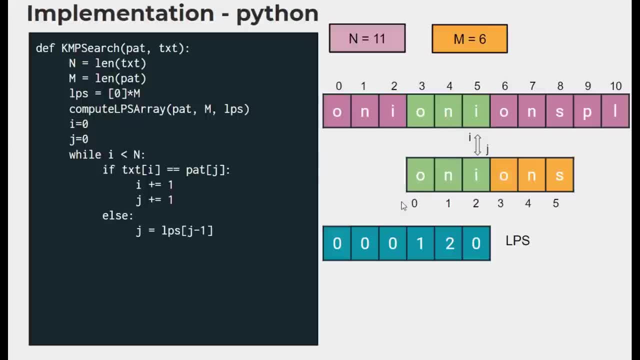 So we can directly start comparing from the second index like this: See, here the value of j is 5 and we now have to go to the fourth index and see what is the value in the LPS table. So that is why we are assigning LPS of j minus 1 as the new j, because this is where we have to. 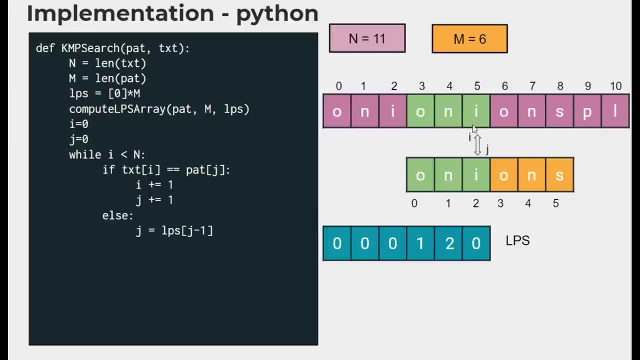 start our next comparison. Notice that i is going to remain the same wherever the mismatch occurred. we are still in the same position And we just have shifted j by looking up the LPS table, Since we are finding LPS of j minus 1,. 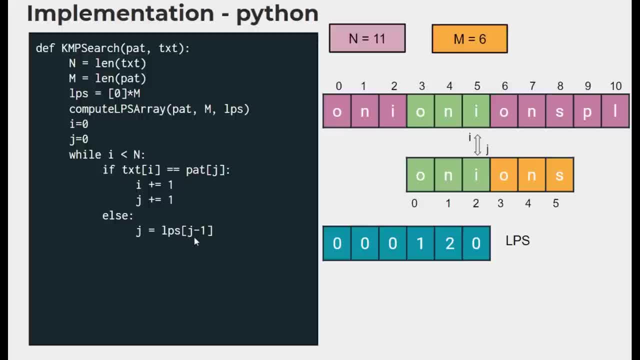 we cannot do that when j is equal to 0, right, If j is 0, that is, if the first character itself does not match, we cannot find LPS of minus 1.. So we can do this only when j is not equal to 0. 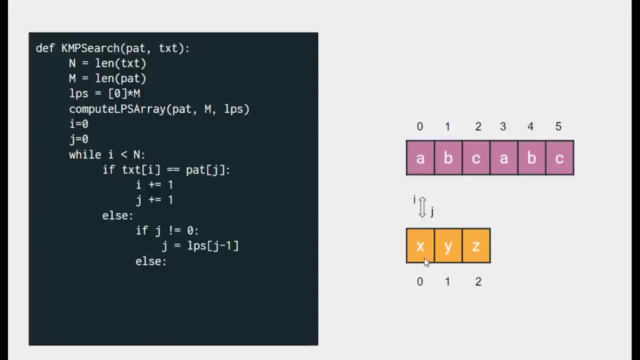 What are we supposed to do when the mismatch occurs when j equal to 0? Take this simple example. Here the mismatch occurs in the first character itself: j is 0. So we just have to go to the next character in the text, right? We just have to increment i and j remains the same. So that is. 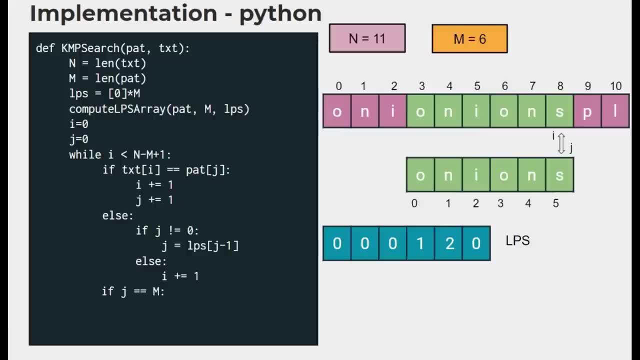 what we are doing here. Again, coming back to this example, if all the characters have matched j will be equal to m, the length of the pattern. We have progressed until the end of the pattern. So if that is the case, we now have to print what is the occurrence 3? is the starting index right? 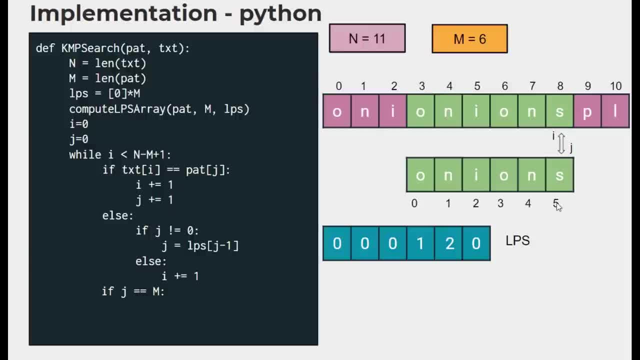 We only know i is 8 and j is 5.. So we just have to print what is i minus j. If you want to continue searching for all the occurrences, we just have to print the length of the pattern. So we just have. 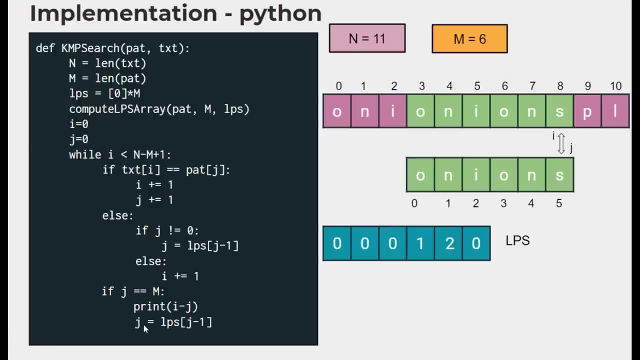 to reset j again to LPS of j minus 1, just like how we did here. We simply cannot search from this point. There might be some overlap here as well. That's why we reset j to LPS of j minus 1 and. 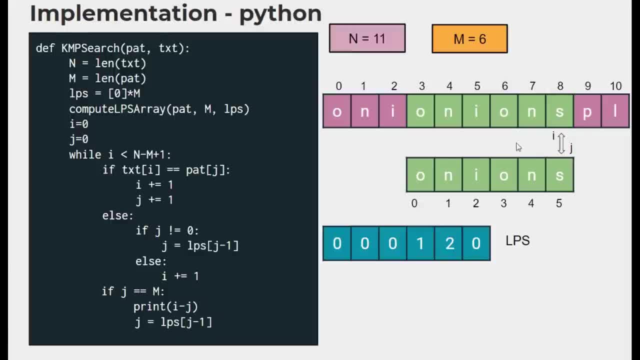 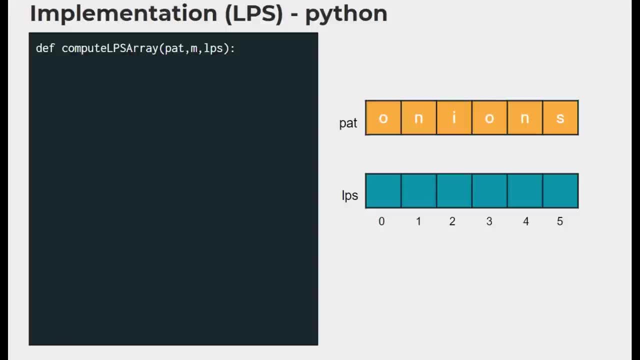 continue searching further till the end of the text input, Coming to the implementation of the LPS array. it is almost going to be same as what we did in the search function. In the search function we had a text and a pattern. We used two different pointers to match the string. 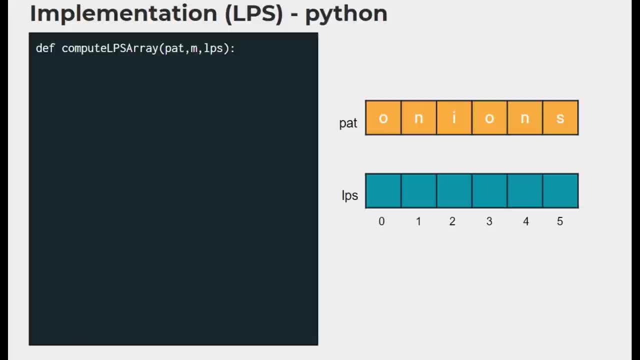 But for the LPS computation we only have the pattern. here We are going to make use of two different pointers, But the string matching has to be done within the pattern itself. We are going to make use of this i to progress till the end of the pattern, And this length is going to actually tell. 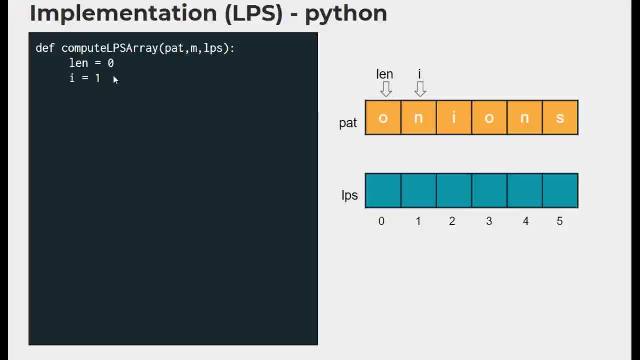 us the length of the matching prefix. that is also a suffix. To begin with, we can initialize length as 0 and i as 1.. LPS of 0 will always be 0, because if you consider only the first character, o, there is no prefix or suffix there. Here the length of the prefix is 0 and i is 1.. So we can. 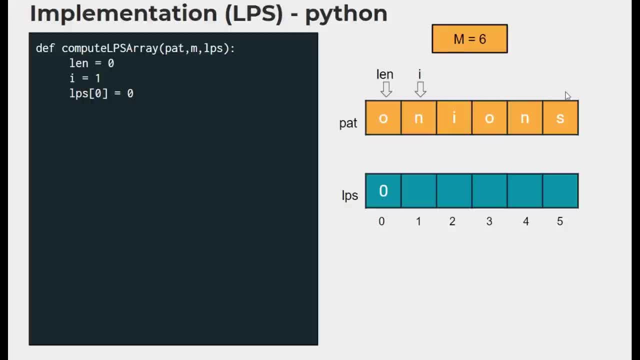 assign length of the prefix as 0 and i as 1.. So we can assign length of the prefix as 0 and i as 1.. So while i is less than m, first we compare these two positions. So when you are computing the LPS of i, 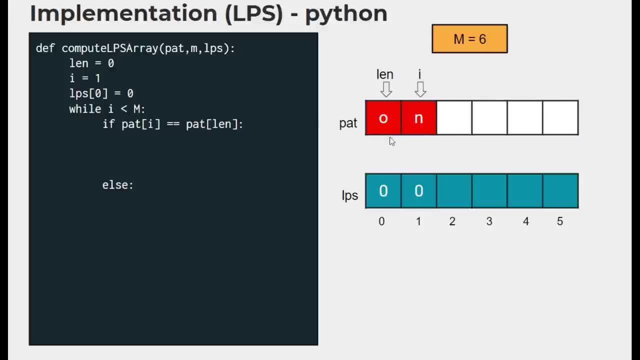 just forget about anything that is beyond i. Just by looking at this string, we can see that we should get a 0 here, because there is no prefix, that is also a suffix and there is a mismatch during the comparison, right? So when we have a mismatch, let's write the else part first. 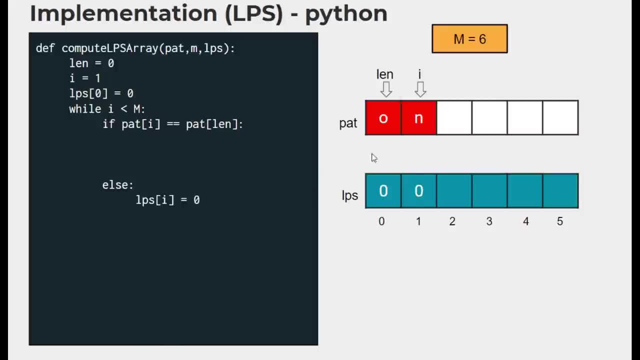 In this case we have to assign LPS of i as 0 and we want to have to increment i here Without finding a match. we cannot increment length right. We are finding the length of the prefix, So it should start from here Only if there is a o. 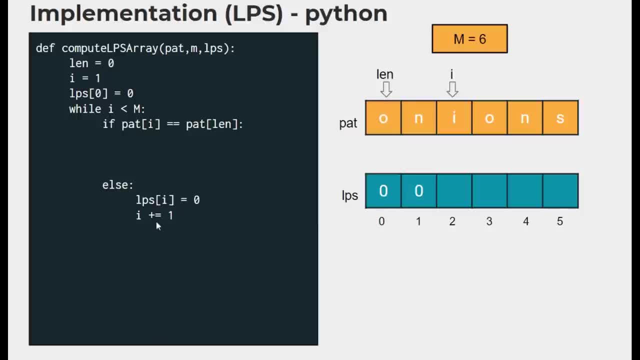 then we can increment length. So we just increment i in this step and now again compare these two characters. Again, there is a mismatch. We already have a code for mismatch. This will get executed and we will have a 0, which is correct. Now we can again increment i to compare. 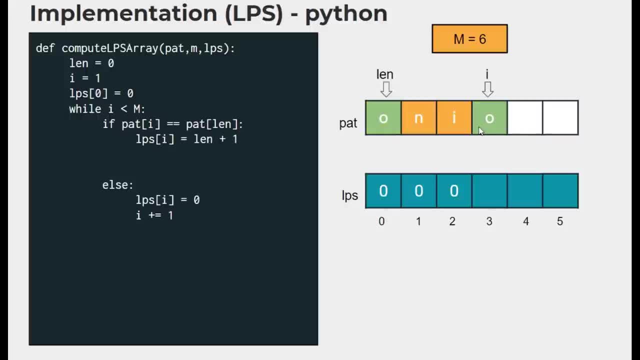 these two characters. now We have a match here. Now the length should now be assigned as 1, right, The length pointer is still at 0, but now the 0th index is a match. So we are adding 1 to that and then assigning to LPS of i, because array index will. 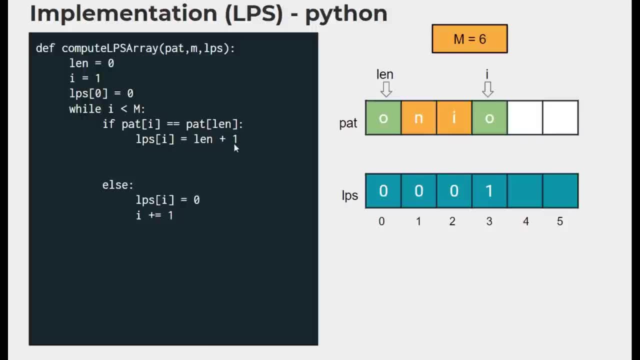 always be 1 behind in the count right. So that is why we are adding 1 and then assigning it to LPS of i. Now, since there is a match, we have to increment both the pointers, So we just increment. 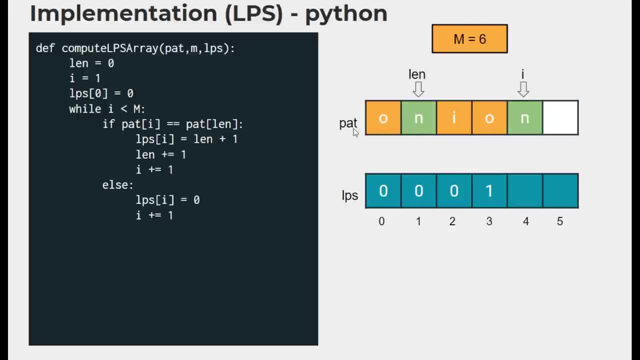 the length and i. These two characters match, So this code will be executed and we will assign to LPS of i. Length is now 1.. So 1 plus 1 is 2 and it is correct because the length of the longest. 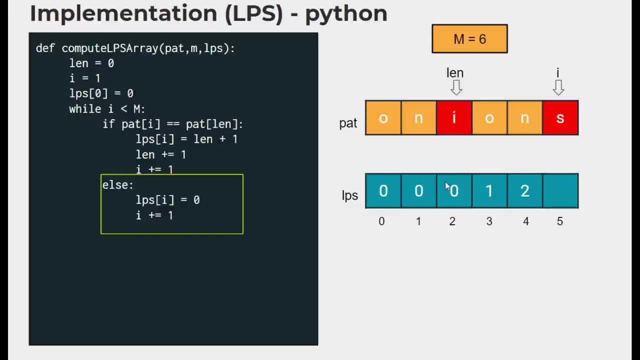 prefix, that's also a suffix- is actually 2, and again we increment both the pointers. Now there is a mismatch. So we just put a 0 here and increment i and we reach the end of the string. So that's it. We have computed the LPS and it seems to be correct, but the else part here needs. 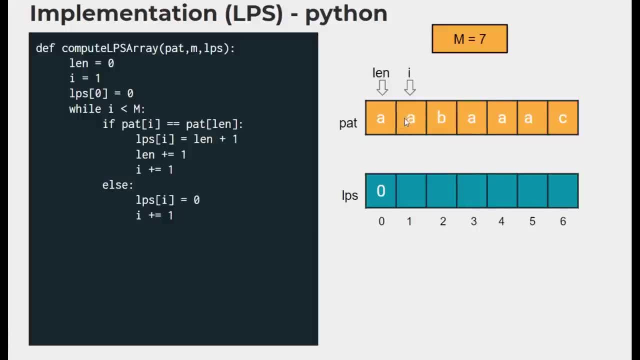 some changes. We will see why with a different example Here. in this example we first put a 0 in 0th index of the LPS and we now compare these two positions. They match. So when they match, what we have to do? Just assign length plus 1 as the LPS of i. So here we put 1 and increment. 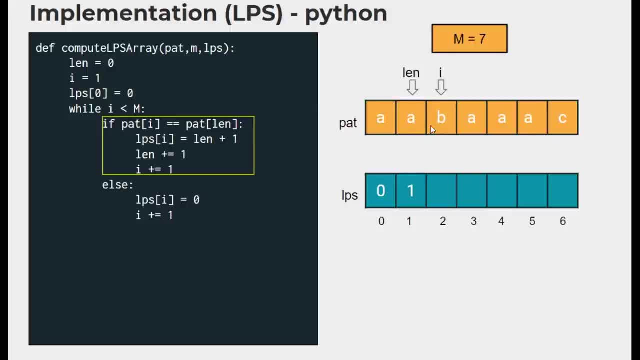 both the pointers. Now, when we compare these two, there is a mismatch. So when there is a mismatch, according to our code, just put a 0 there and increment. i Just think, can I compare this and this? now Does it make sense? Already there was a mismatch here, which means we have. 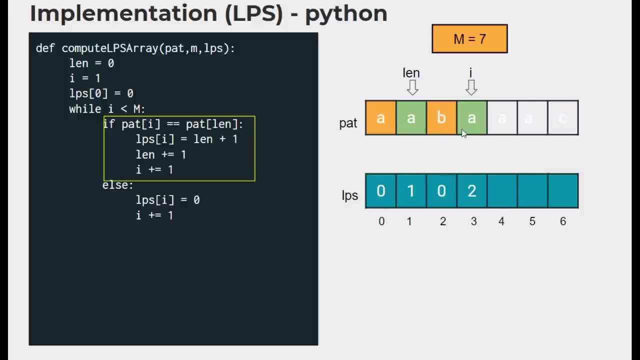 lost the continuity. Say, for instance, we go by this code and compare these two positions, We have a match and as per this code, length plus 1 will be 2 and we cannot put a 2 here. It is wrong In this substring there is no prefix. that is also a suffix of length 2.. We only have a and a here. 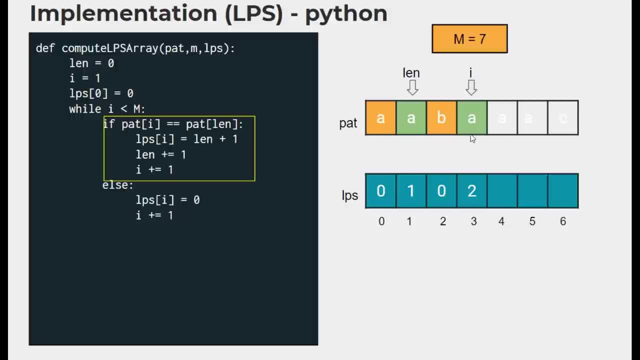 So the length of the prefix that is also a suffix is of length 1 only. So whenever a mismatch like this occurs and if we have already progressed in length, we have to go backward in direction right, Otherwise we will lose the continuity. If we are still in the first position of the pattern, the length. 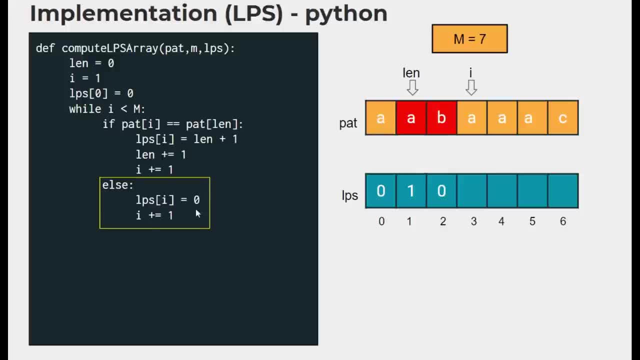 is in the first position of the pattern, then we can go by this code. It will work. That is why it worked for our previous example. But if we have progressed in length, we cannot go by this code. So when this length pointer is not equal to 0, we now have to think what is the new position for? 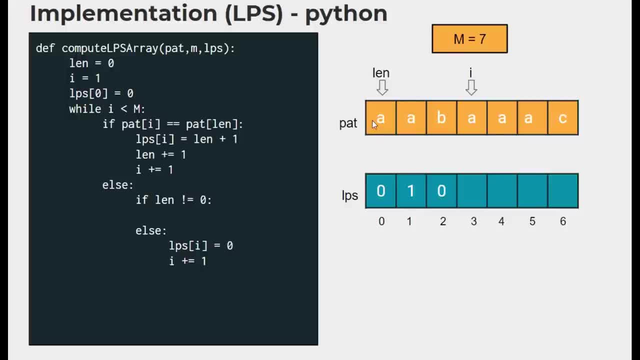 this length pointer, We would intuitively think to go all the way back and start from the beginning, that is, assign length as 0 and then continue on. So this is our search, but again this will not be correct. Let's see why. Let's just continue with. 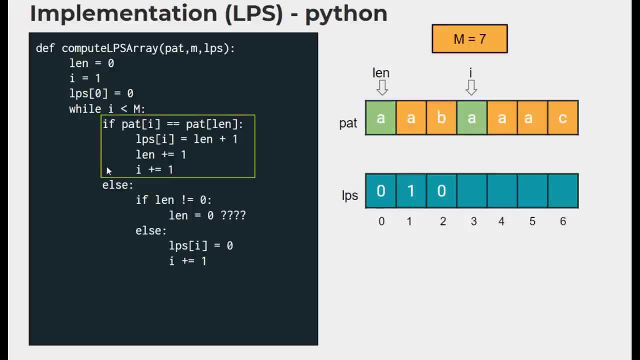 this code. On comparing these two, there is a match, So this code will be executed. Length is now 0.. So when we add 1, we get a 1 here, and it is correct. We increment both the pointers On. 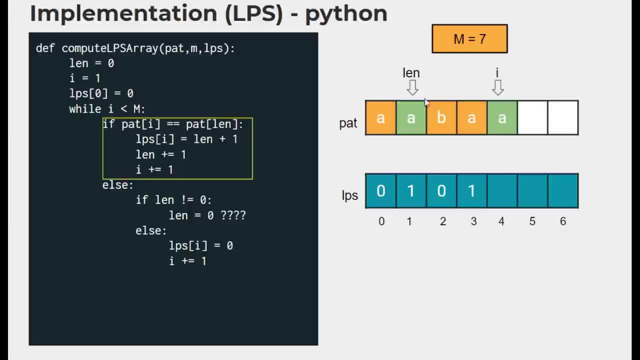 comparing these two again, they match. Length plus 1 is 2 now and it is correct, because now the length of the prefix that is also a suffix is of length 2 and our code is working properly. Now, when we increment both the pointers and compare these positions, there is a mismatch, Since length is. 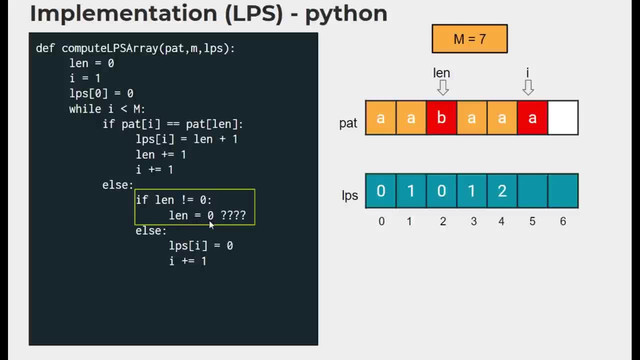 not equal to 0,. according to this code, we set length as 0 and again compare these two positions. Based on this code, we will put a 1 here, but that is not correct. Just observe this substring carefully. The length of the longest prefix, that is also a suffix, is of length 2, right. 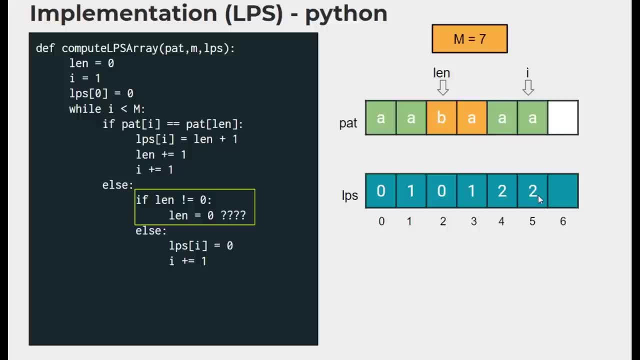 aa, aa. So actually we need a 2 here and not 1.. What is the problem here? Let me bring this part down so that now you can see this is going to be exactly the same scenario that we discussed for the search method. When there is a mismatch here, we know that this and this match Actually. 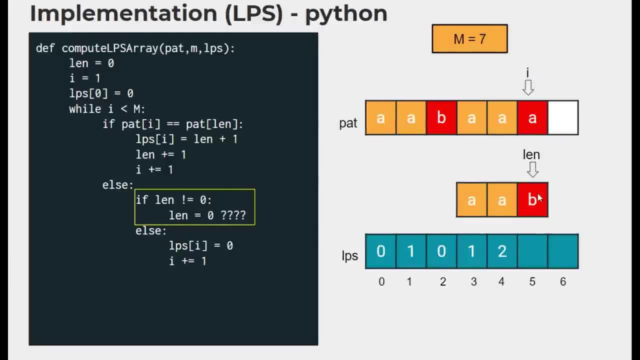 this is present here, Just because there is a mismatch here. we cannot start all the way from the beginning, right? But that is what we are doing here by assigning length as 0. This a has to overlap with this a and we have to actually compare this i with the first position. But how? 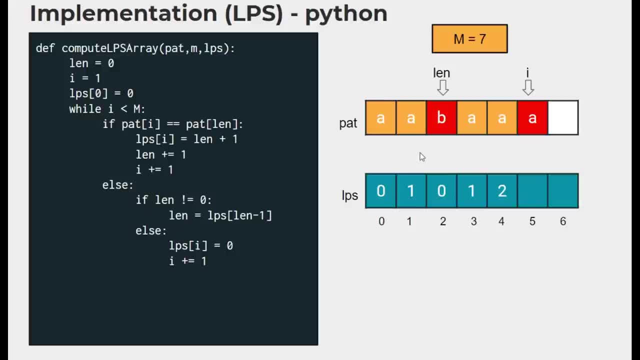 do we know how many characters are there in the first position? We have to know how many characters are there in the first position. We have to know how many characters are there in the first position. We have already computed the LPS until this point right, So we just have to assign LPS of length. 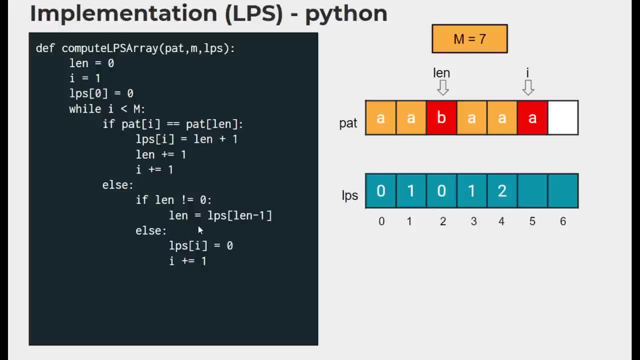 minus 1 as the new length and then continue Just like how we did for the search method. LPS of length minus 1 is now 1.. So we just have to reset length to this position and then compare: They match. So, as per this code, we can put a 2 here and increment both the pointers. 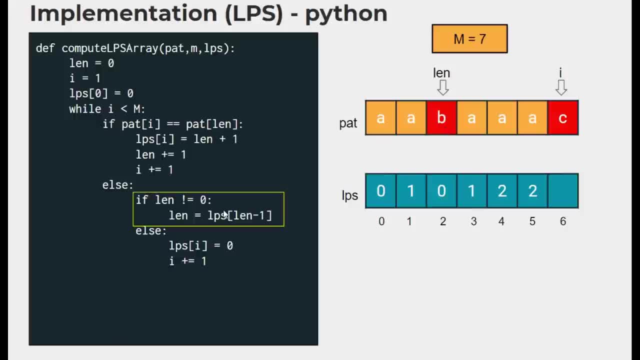 And now there is a mismatch and length is not equal to 0.. We again have to check if there is a overlap. So we assign LPS of length minus 1 as the new length and compare at this position. now Again there is a mismatch. So we go to this position 0 and compare. There is a. 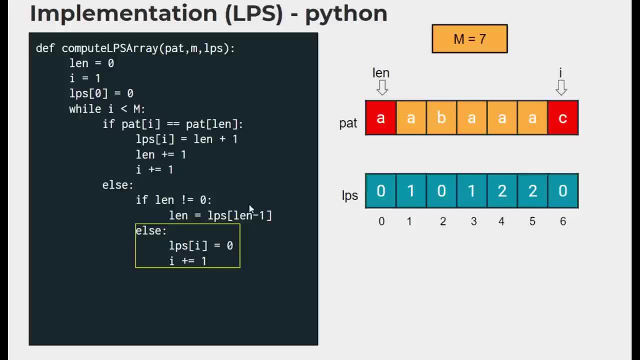 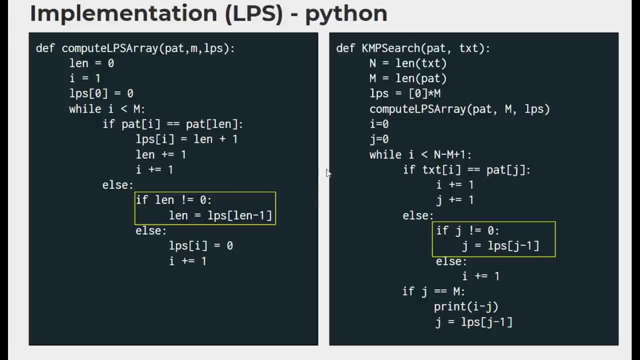 mismatch. So we can put a 0 now, since length is equal to 0.. We execute this part of the code. We have both the methods that we discussed: LPS and the search method. If you see, here it is the same logic. Here in the LPS computation it is just a single. 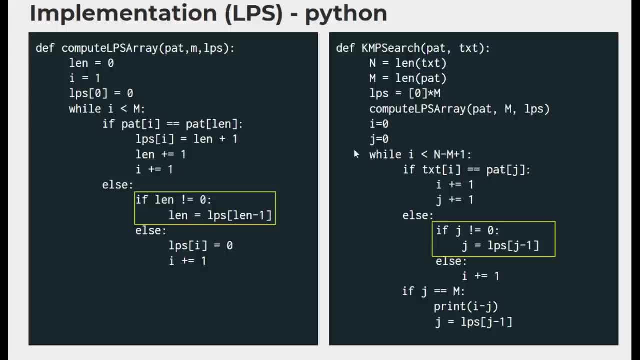 array, but here we have two arrays. That is the only difference. Since this is one single array, it might seem little confusing, but if you compare these two, then you can easily understand the logic. Moving on to the time complexity, we know that the text pointer that we used in the KMP 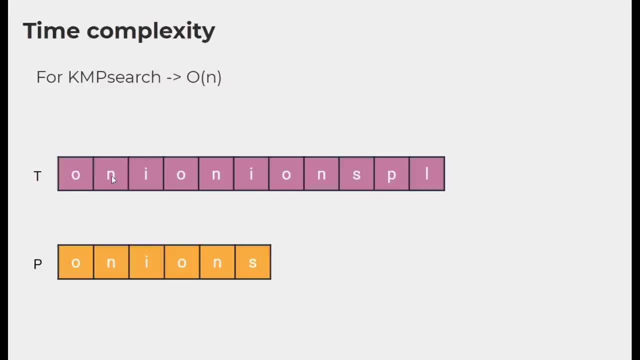 search method never move backwards, which means for each and every character present in the text input, we only perform some constant number of operations, including the LPS lookup. Since the number of operations is going to be a constant multiple of n, it can be considered as a O complexity, ie linear time.